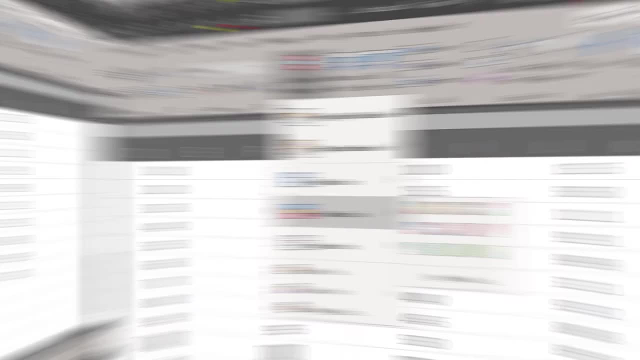 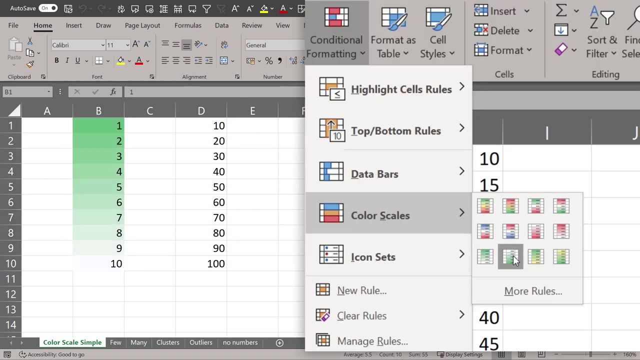 have created earlier. Today we will see color scales. Let's start with simple data. It's just one to ten. You can choose either a two color scale or a three color scale. We will start with a simple two color scale: Yellow to green. How does this work? The minimum number gets one color. 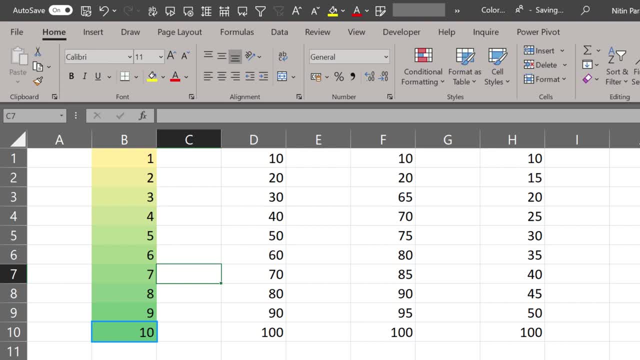 The maximum number gets another color and intermediate numbers get a mixture of two colors. The minimum number gets one color. The maximum number gets another color. If it's nearer to the minimum color, it gets more yellow If it's nearer to the maximum color. 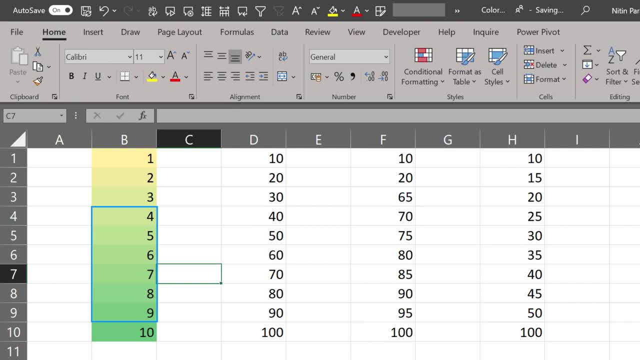 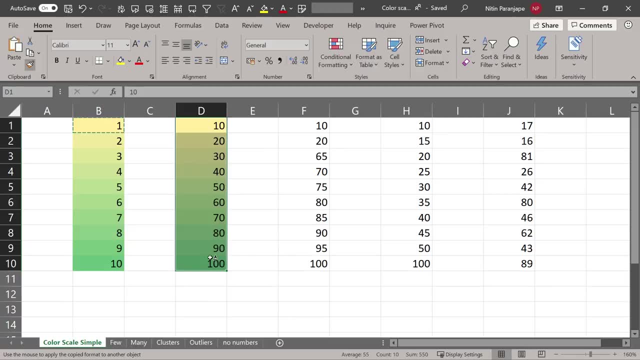 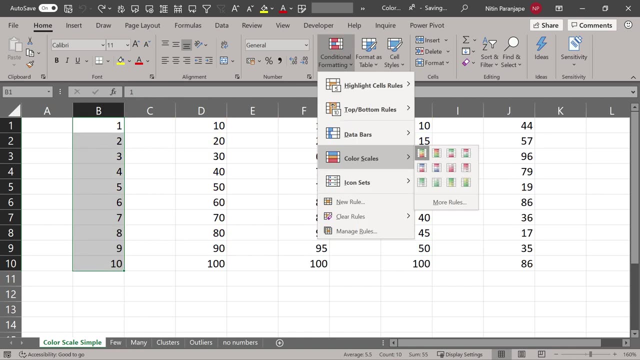 it gets more green. Now let's apply this to different sets of numbers. I want to do format paint multiple times, So I'm going to double click on the format painter. Now you will get a better idea of how this color distribution works. If there was a three. 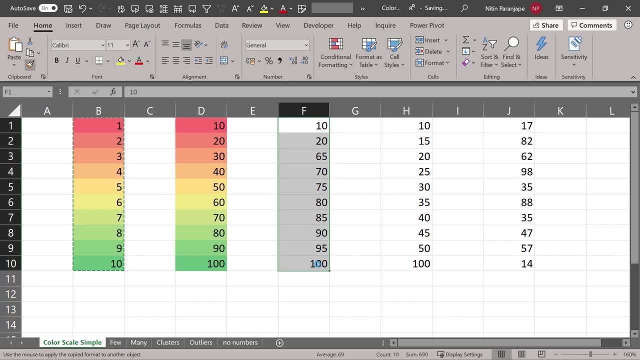 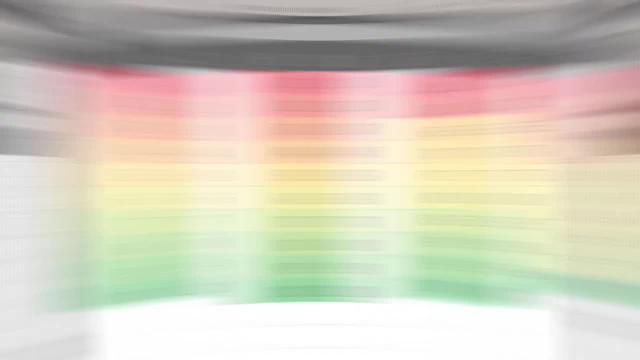 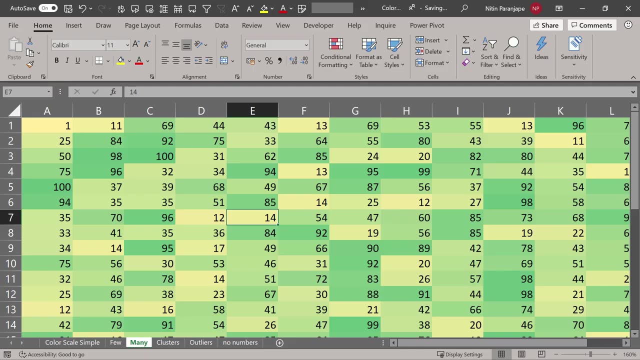 color scale. let me show you how this works. So instead of two boundary colors, we have three colors: minimum, maximum and middle. So if you use it for mixed data, it may or may not be very useful. Even when I applied to large set of numbers, it's still looking jumbled up. So the real value of 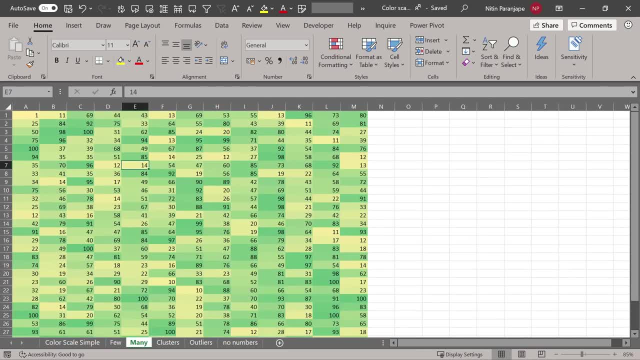 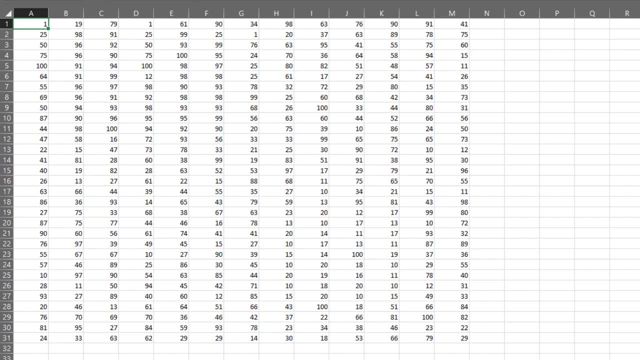 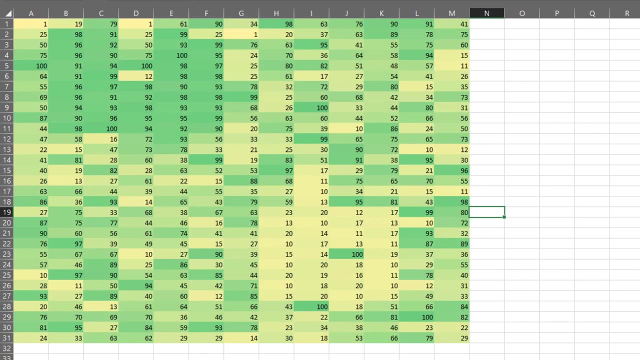 color scale comes. when you zoom out Here, you will clearly see that there is no single pattern. Now. Now let's try it with something else. The data looks similar. It's very difficult to understand how the data is distributed, but when I apply color scale, you will notice that. 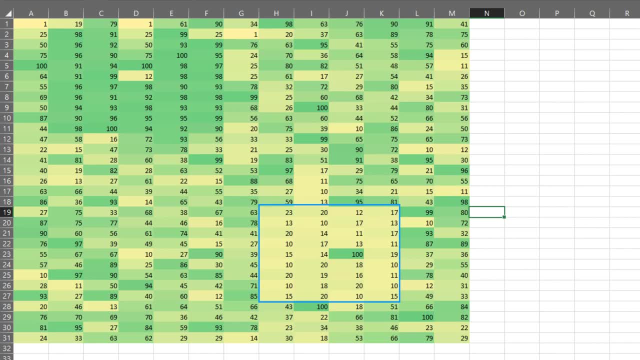 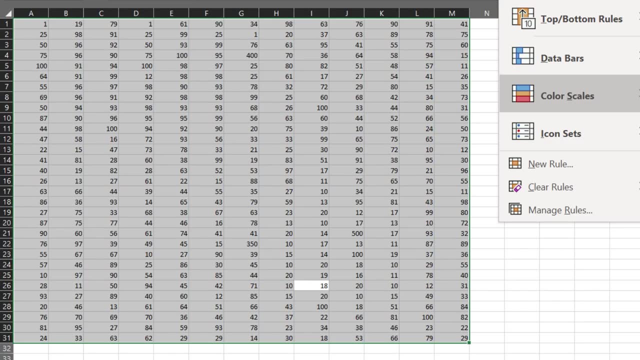 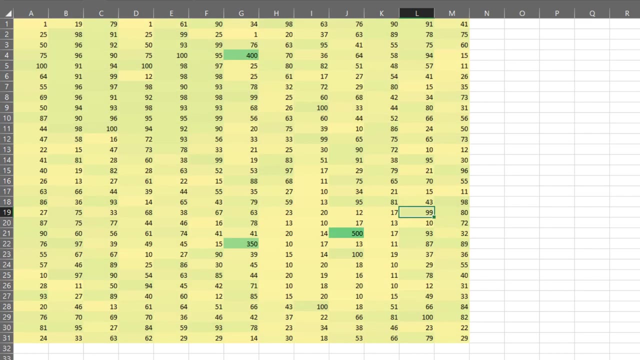 there is a cluster of high values here, cluster of low values here, and you can even see exceptions very clearly here. Another use of color scale is to find abnormally large or small values Using the same color scale, but because some values were. 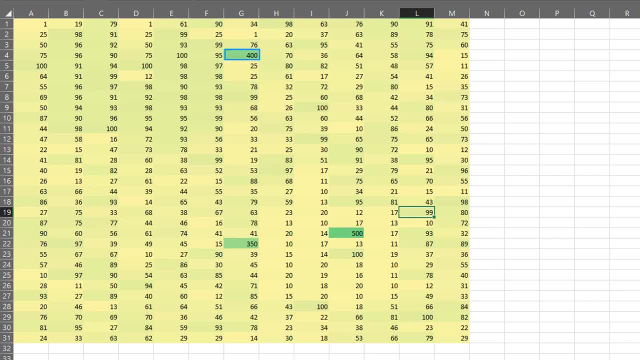 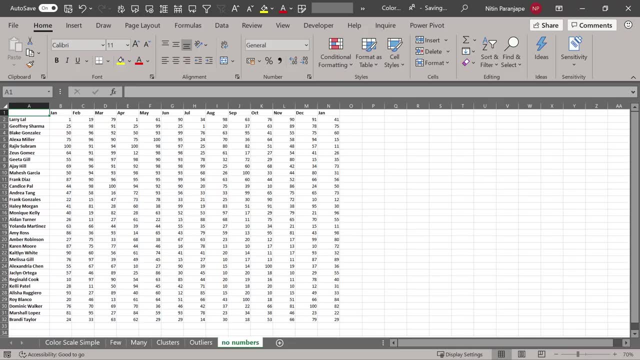 much bigger: 350,, 500, 400, they become green. Everything else is yellowish. That is called outliers. And finally, when you want to show a pattern and not worry about numbers, because anyway those numbers are not readable, In that case apply conditional formatting. 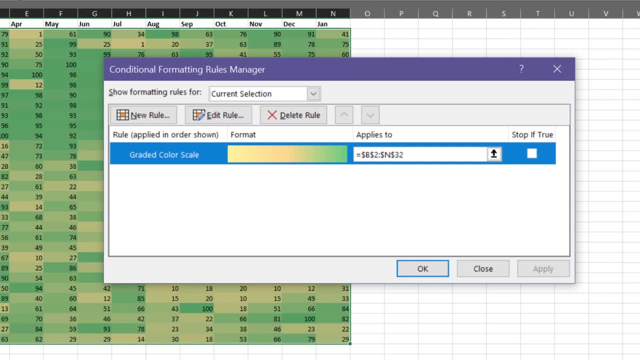 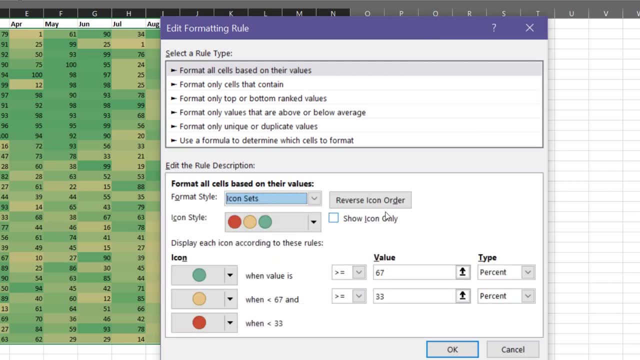 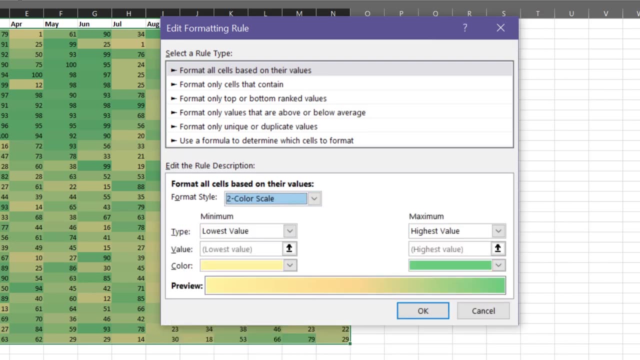 You go to manage rules, edit the rule. Unlike Other types like data bar, which says show bar only, An icon sets, which says show icon only when it comes to color scale, Show color only option doesn't exist. Not to worry, we will do it in a different. 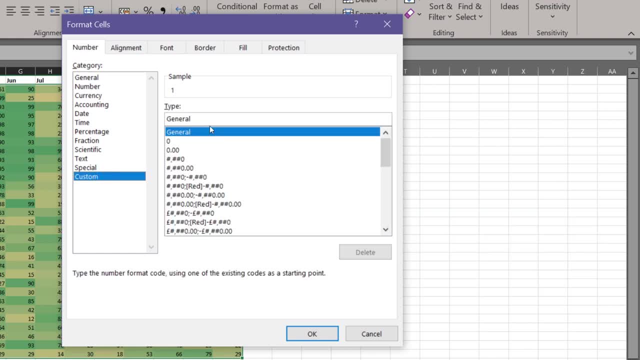 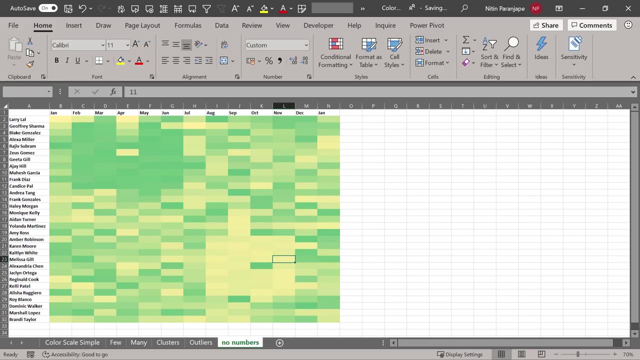 way. So if you go to format cells- this is a shortcut To have a number but not displayed- Put 3 semicolon In the custom formatting. How does this work? Well, That's for another video, But now here you can see how people are performing. 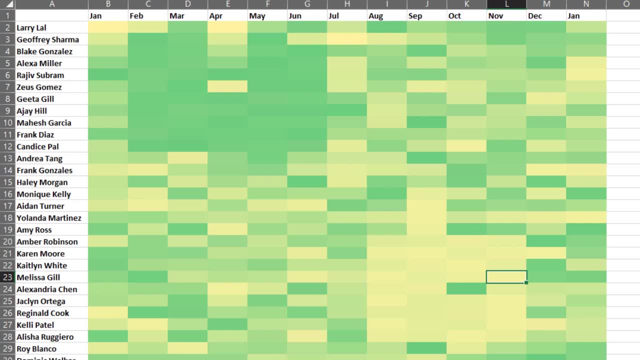 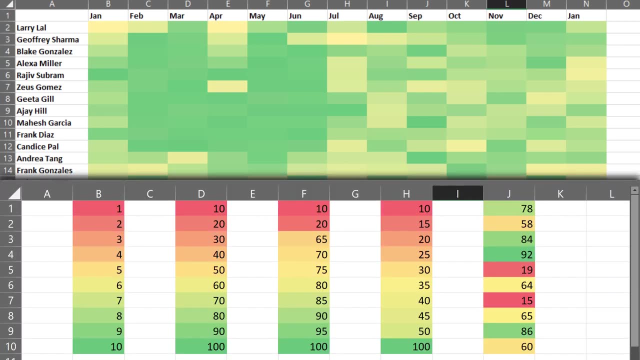 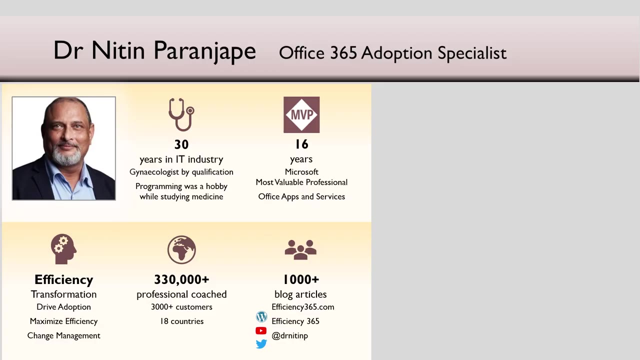 across time without getting confused with individual numbers. Now this can be copy pasted in a PowerPoint presentation for display purpose. That is how you use color scales. If you like this video, do share it with your friends, colleagues and loved ones. Of course, I'm sure you'll subscribe. 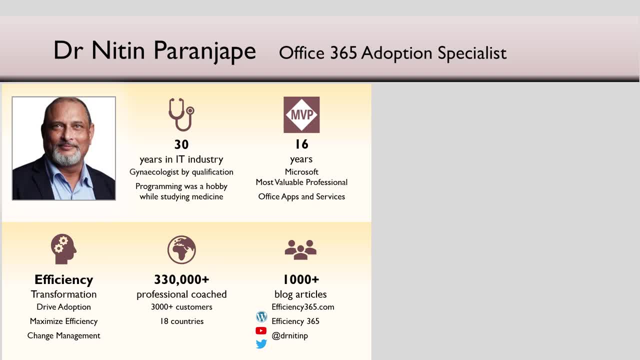 and press the Bell icon. That's all for now. See you very soon with another video. Thank you. 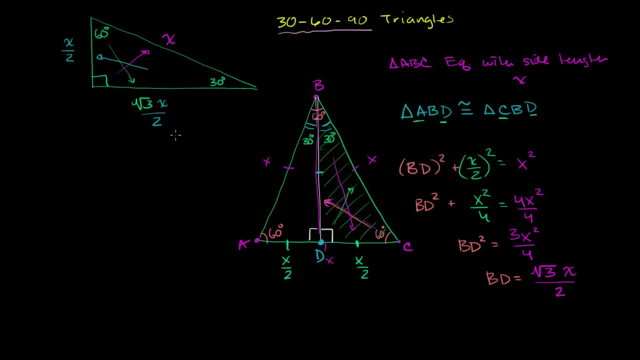 In the last video we showed that the ratios of the sides of a 30-60-90 triangle are: if we assume the longest side is x, if the hypotenuse is x, then the shortest side is x over 2.. 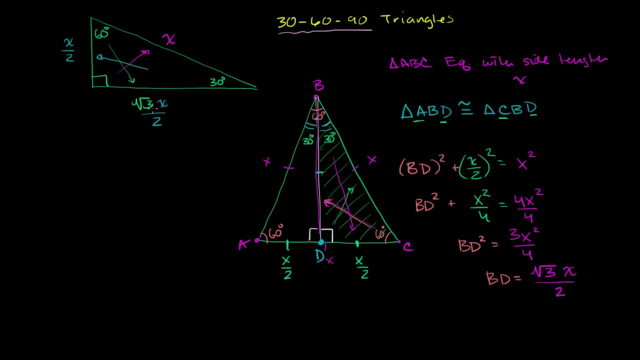 And the side in between, the side that's opposite, the 60-degree side, is square root of 3x over 2.. Or another way to think about it is: if the shortest side is 1, and I'll do the shortest side- then the medium side. 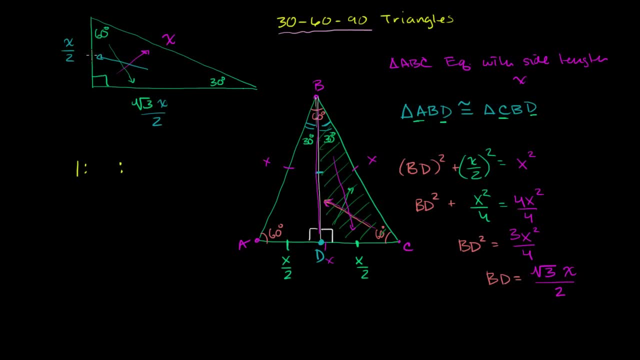 then the longest side. So if the side opposite, the 30-degree side, is 1, then the side opposite, the 60-degree side, is square root of 3 times that. So it's going to be square root of 3.. And then the hypotenuse is going to be twice that. 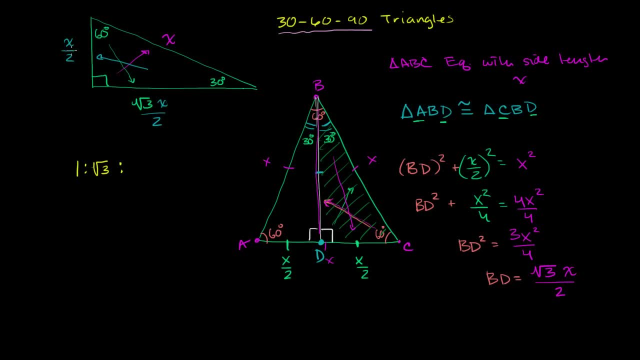 In the last video we started with x and we said that the 30-degree side is x over 2.. But if the 30-degree side is 1, then this is going to be twice that, So it's going to be 2..